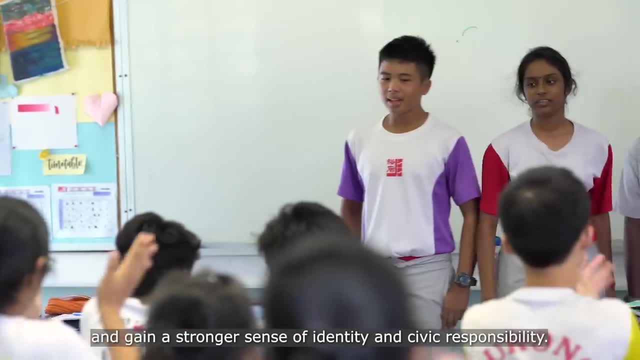 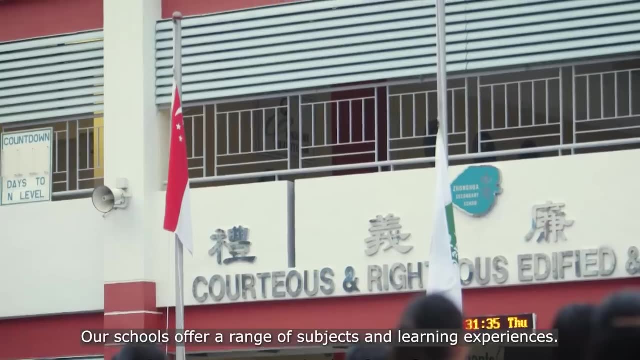 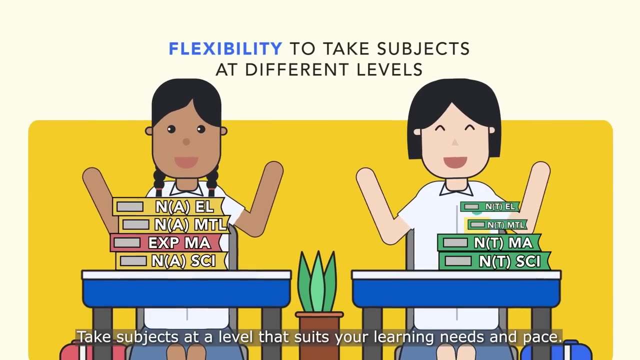 think critically, contribute actively and gain a stronger sense of identity and civic responsibility. Our schools offer a range of subjects and learning experiences. You can customize your learning. Take subjects at a level that suits your learning needs and pace. Make new from all walks of life. 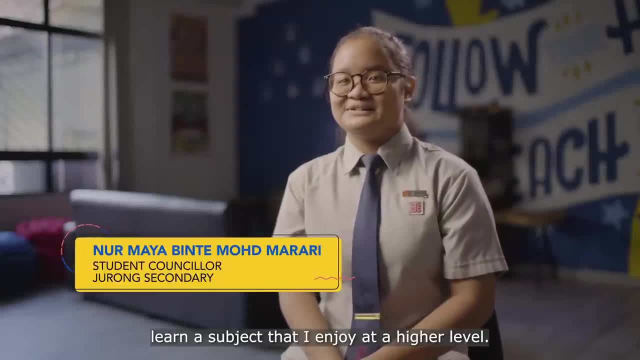 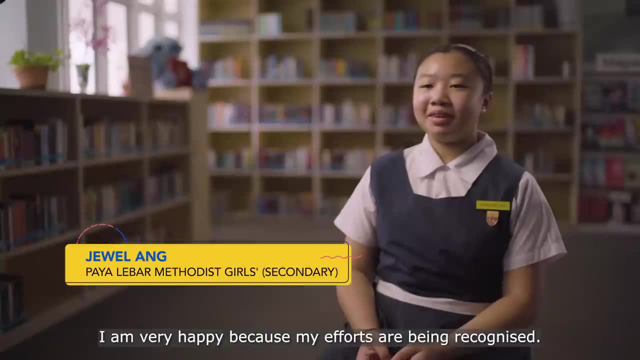 FSBB is an opportunity for me to learn a subject that I enjoy at a higher level. It helps to build my self-esteem Taking subjects at a higher level. I am very happy because my efforts are being recognised. I also get to make more new friends. 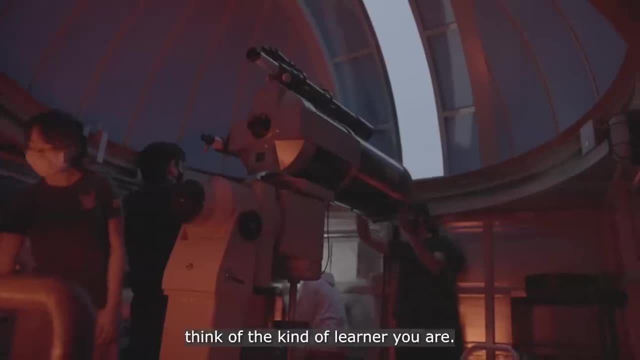 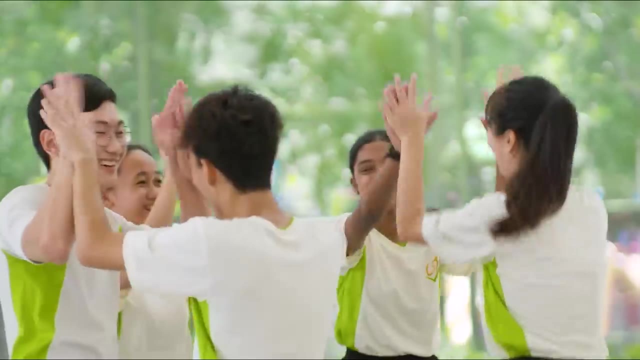 As you consider your secondary school options, think of the kind of learner you are. What are you good at? Are there subjects and skills that you would like to explore If you enjoy a more practical and hands-on way of learning and a more customised curriculum? 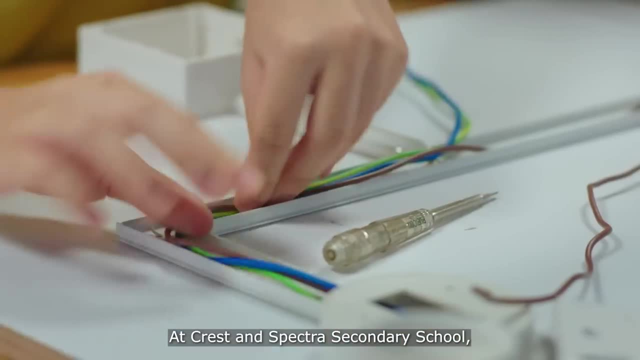 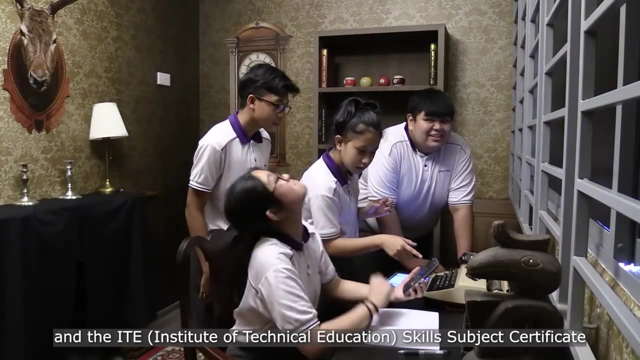 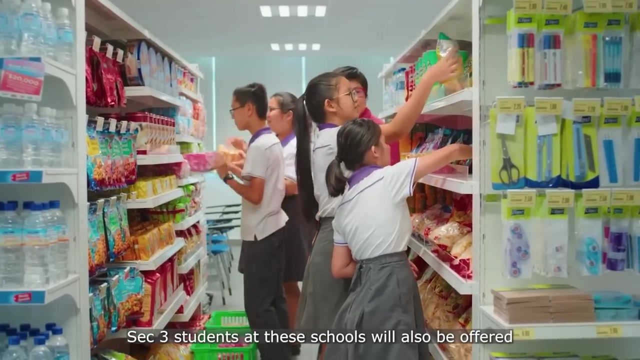 you can consider one of the specialised schools. At Crest and Spectra Secondary School you will graduate with a combination of GCE N-Level and the ITE Skills Subject Certificate at the end of Sec 4.. Sec 3 students at these schools will also be offered the ITE Skills Subject Certificate. 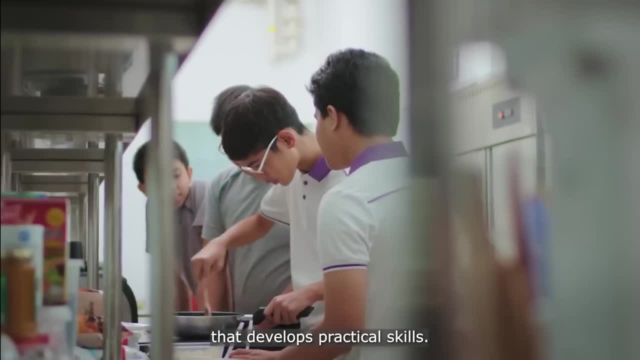 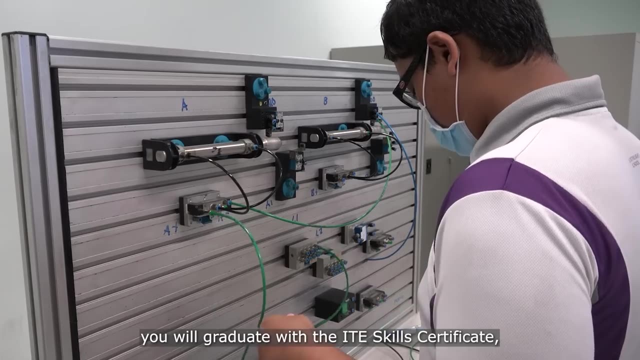 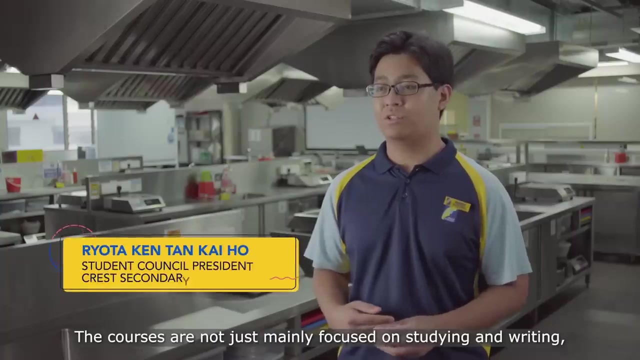 which has a broad-based curriculum That develops practical skills. At Northlight School and Assumption Pathway School, you will graduate with the ITE Skills Certificate, which prepares you for employment or admission to ITE. The courses are not just mainly focused on studying and writing, but also focused on hands-on. 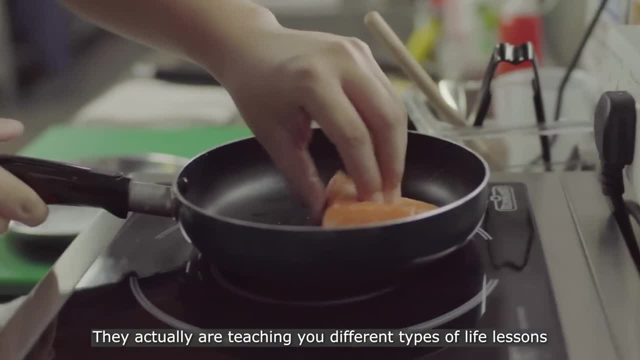 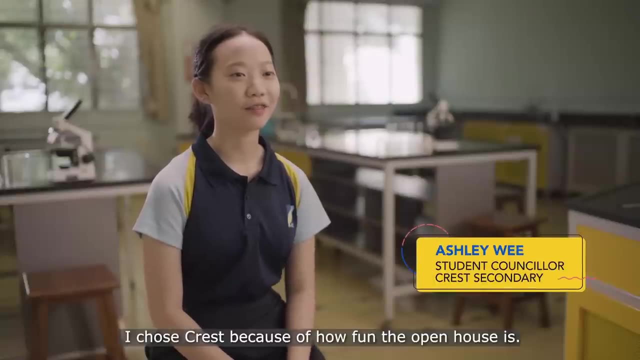 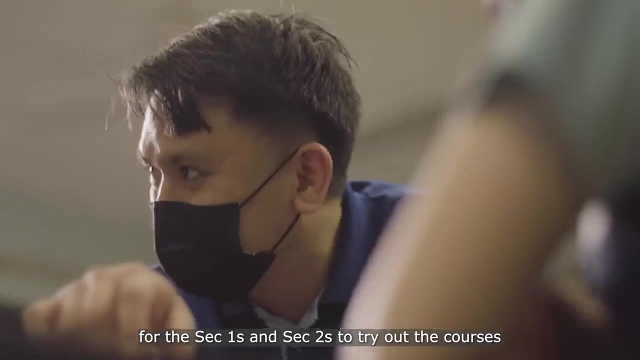 such as cooking, mechanical design. They actually are teaching you different types of life lessons and what you can do in the future. I chose Crest because I love how fun the open house is. The TASTER module is a programme that we have for the Sec 1 and Sec 2. 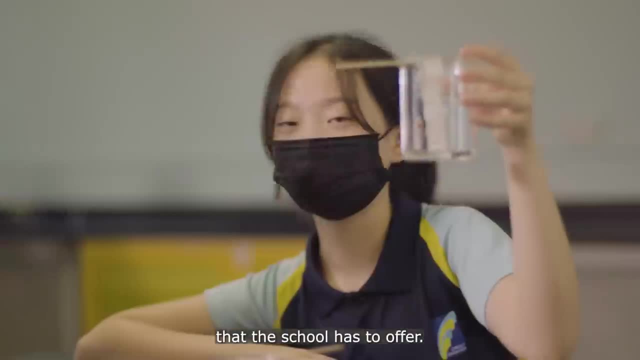 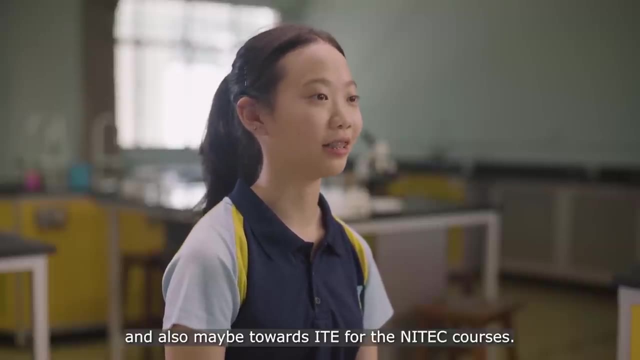 to try out the courses that the school has to offer so that we can continue learning in Sec 3 and Sec 4, and also maybe towards ITE for the NITEC courses, If you have a promising talent and keen interest in a specific area. 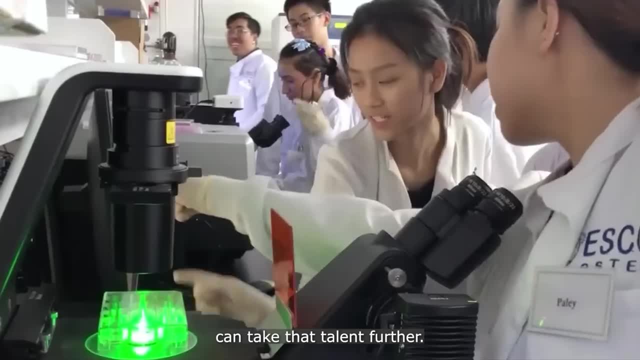 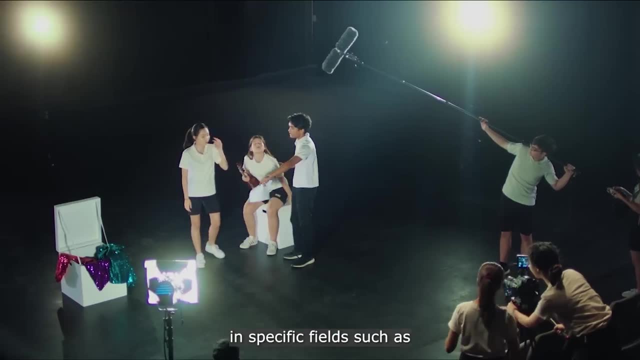 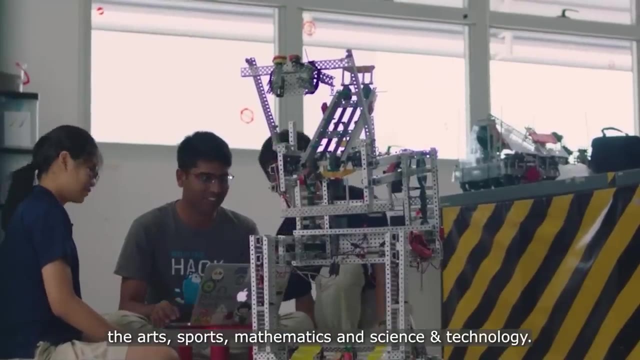 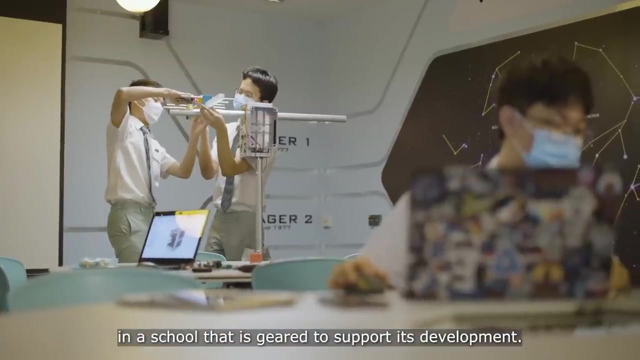 our specialised independent schools can take that talent further. On top of a general curriculum, these schools focus on developing students in specific fields such as the arts, sports, mathematics and science and technology. Expect to spend more time and effort on your specific strength in a school that is geared to support its development. 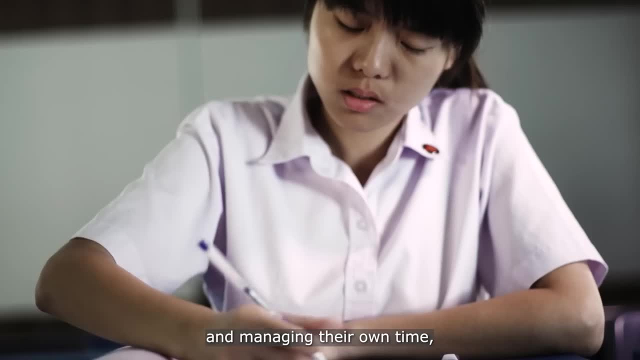 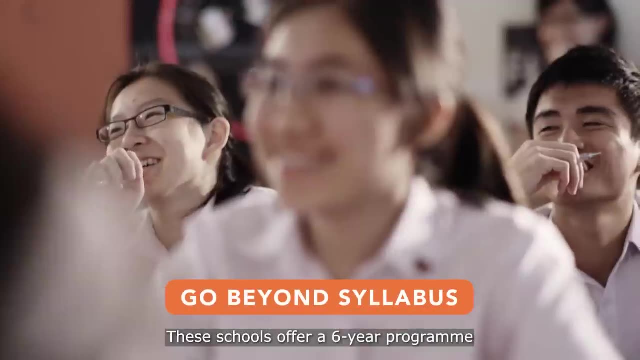 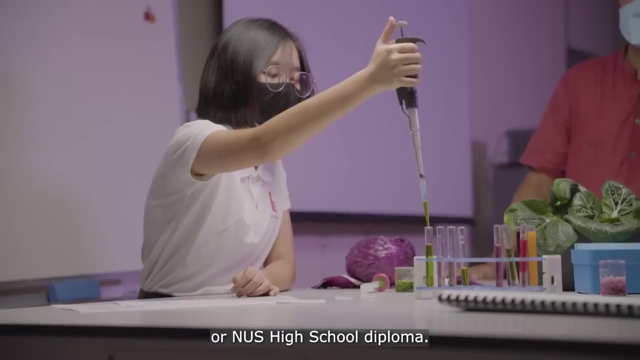 Those who like independent learning and managing their own time can consider the integrated programme offered in some schools. These schools offer a six-year programme leading to an A-level qualification, International Baccalaureate Diploma or NUS High School Diploma. In these programmes, students immerse themselves in broader learning experiences. 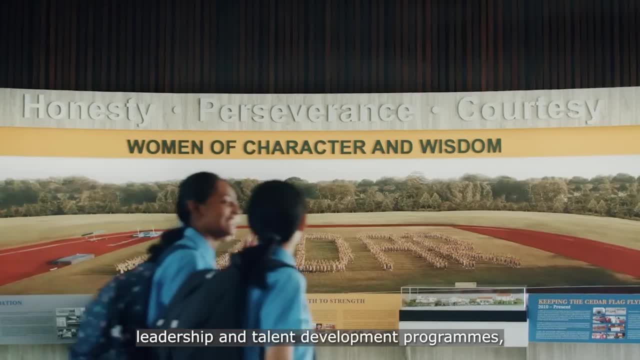 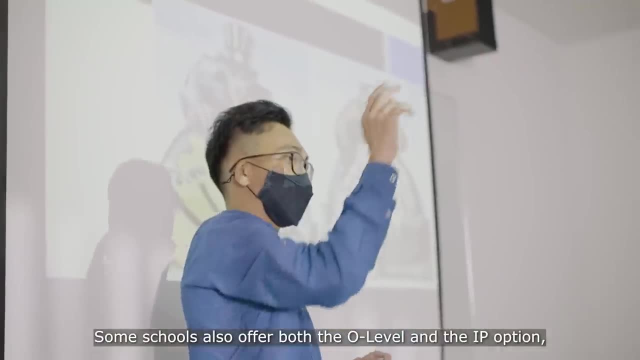 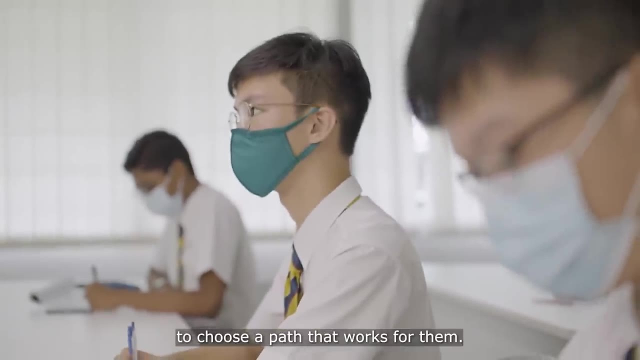 that may include leadership and talent development programmes, work attachments, interdisciplinary learning opportunities and more. Some schools also offer both the O-Level and the IP option, which provide greater flexibility for students to choose a path that works for them. I think the main strength of the IBDB programme is that it really gives the opportunity for us as students. 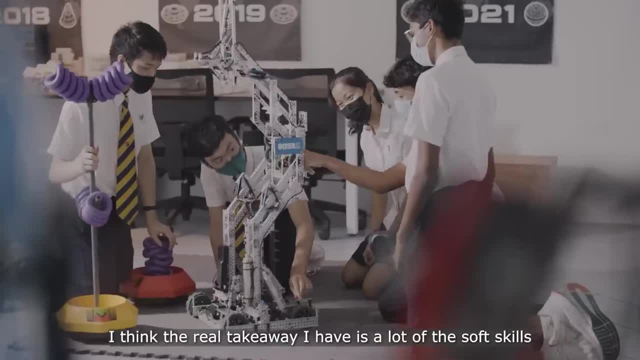 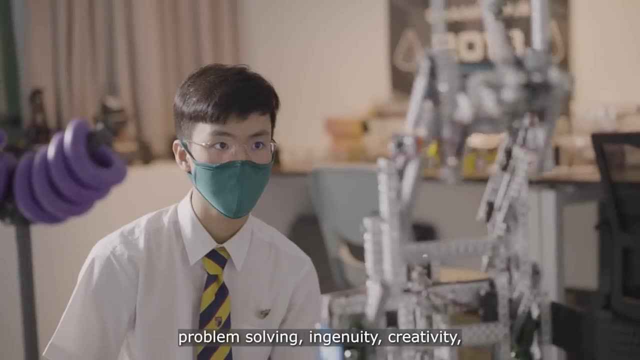 to have a kind of independent learning. I think the real takeaway I have is a lot of the soft skills. like from robotics, I pick up skills like teamwork, problem solving, ingenuity, creativity, coming from very different angles and working hard. 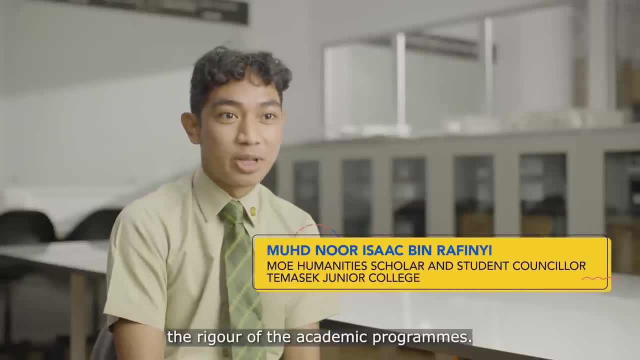 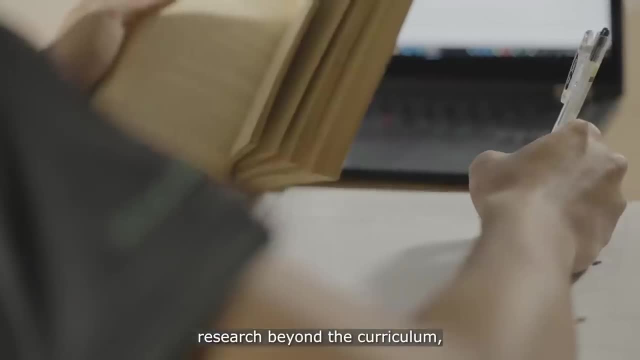 One of the things I enjoyed being in IB was the rigor of the academy programmes. One of the things I enjoyed being in IB was the rigor of the academy programmes. I had the opportunity to participate in all of these stretch programmes, research beyond the curriculum and have hands-on activities. 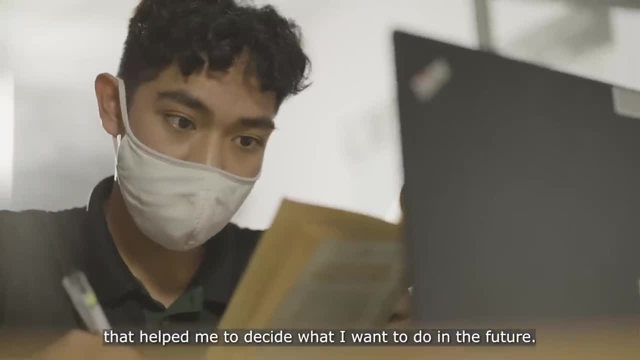 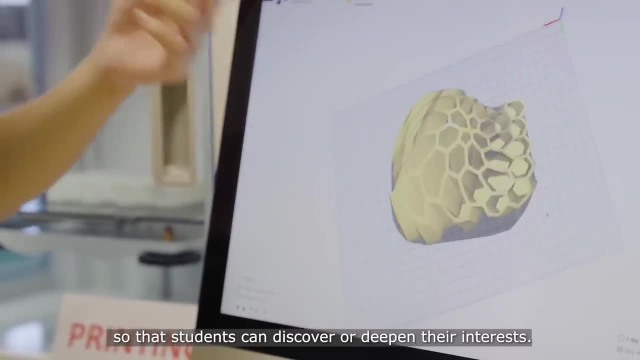 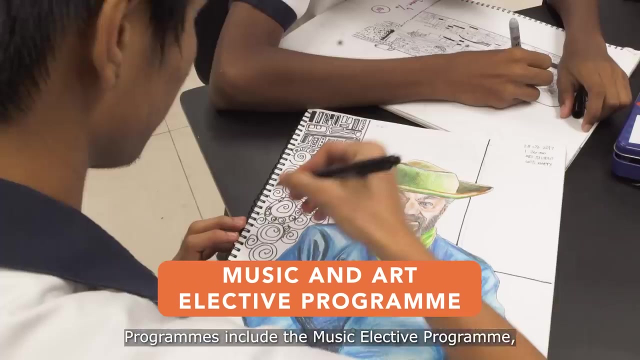 that helped me to decide what I want to do in the future. All our schools offer a wide range of programmes so that students can discover or deepen their interests. Programmes include the Music Elective Programme, Art Elective Programme, as well as various language programmes. 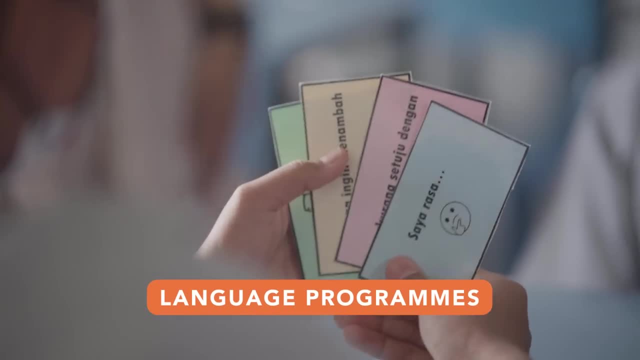 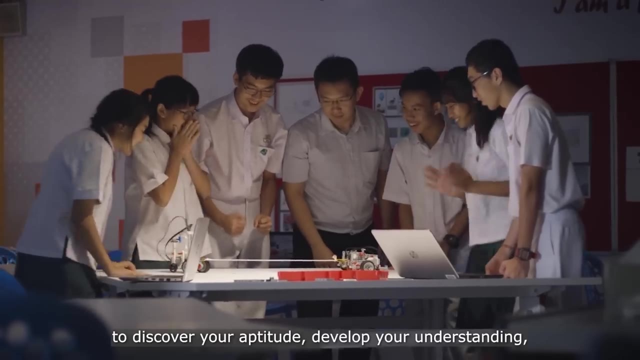 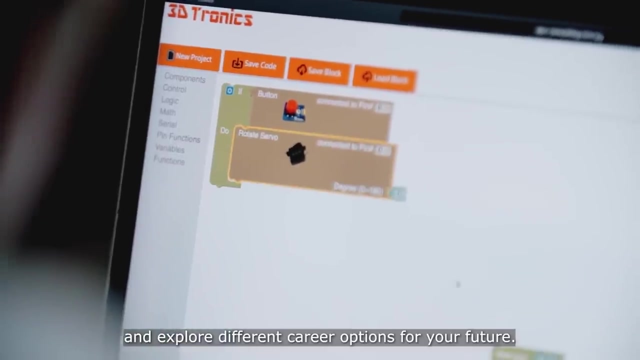 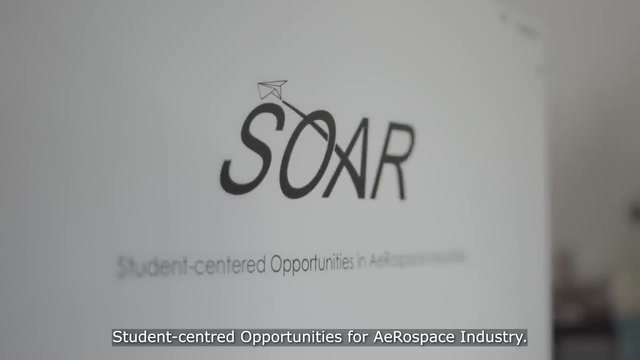 as well as various language programmes, All schools offer applied learning programmes that provide hands-on, real-world opportunities to discover your aptitude, develop your understanding and explore different career options for your future. My ALP programme is titled SOAR: Student Centred Opportunities for Aerospace Industry. 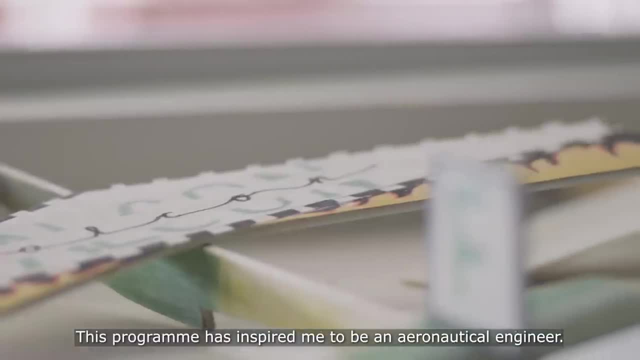 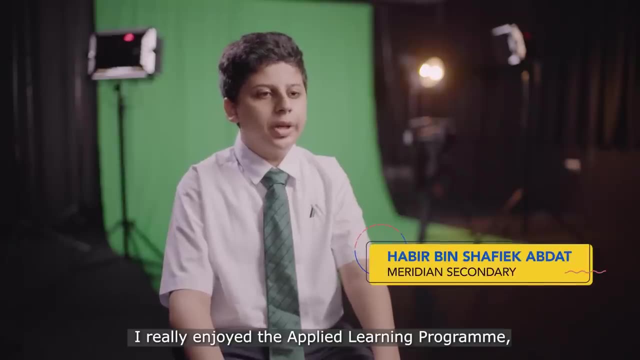 My ALP programme is titled SOAR: Student Centred Opportunities for Aerospace Industry. This programme has inspired me to be an aeronautical engineer. It deepens my understanding and interest in aviation. I really enjoy the applied learning programme as it's a new experience for me to write a book. 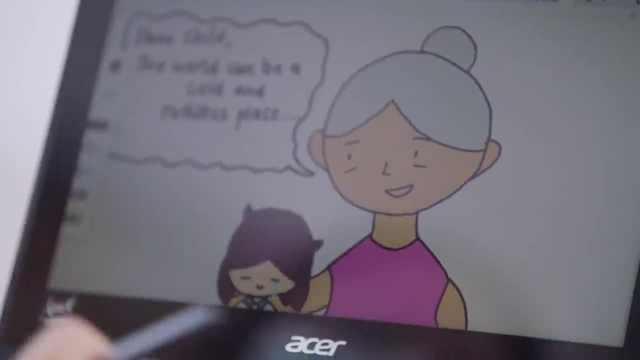 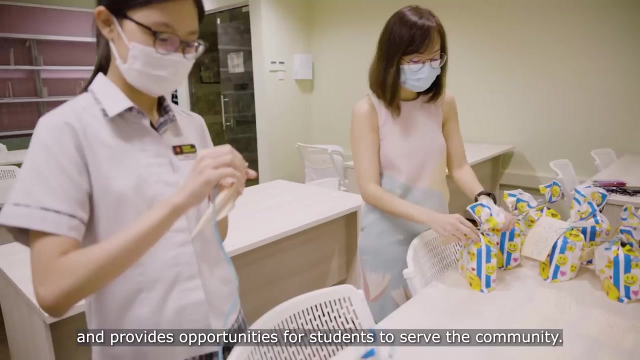 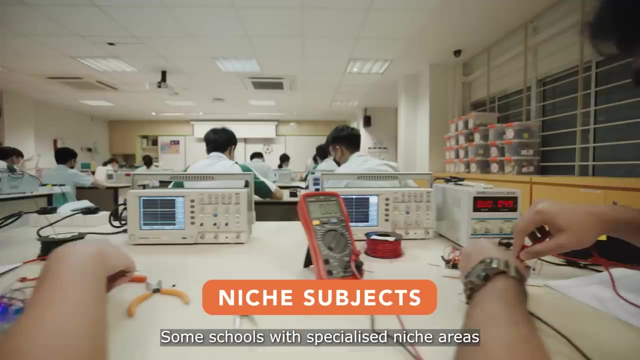 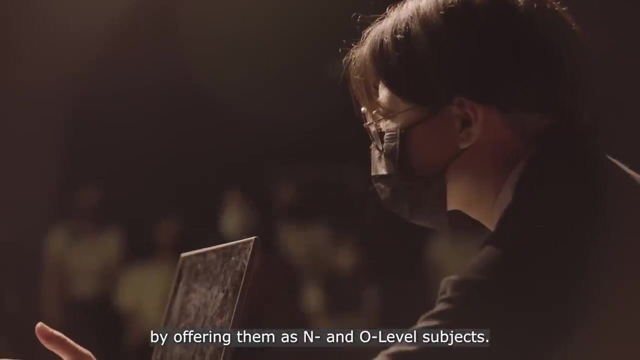 and also how to catch digitally. All schools also offer a Learning for Life programme, which develops students' values and life skills and provides opportunities for students to serve the community. Some schools with specialised niche areas allow you to take your interests further by offering them as N and O level subjects. 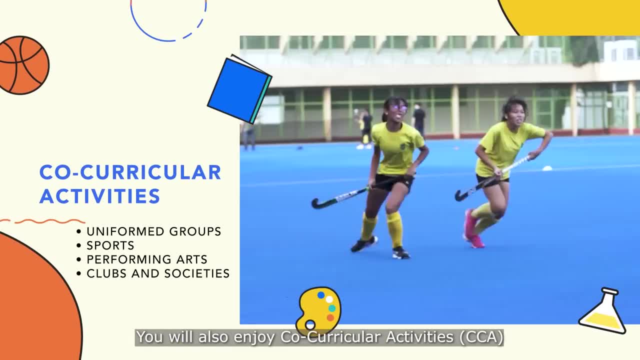 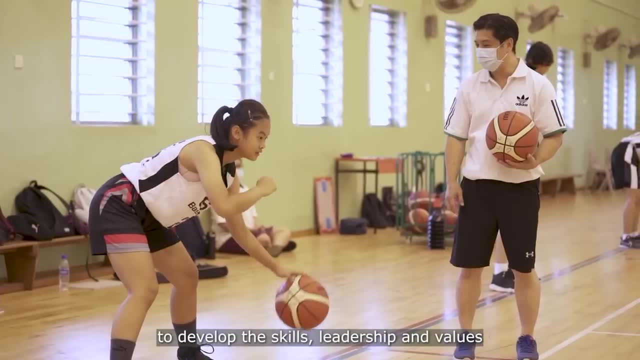 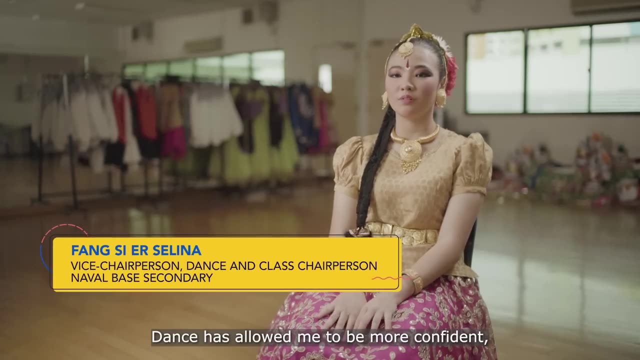 You will also enjoy co-curricular activities. no matter where you go. A wide range of CCAs is offered in each school to develop the skills, leadership and values that cannot be taught in the classroom. Dance has allowed me to be more confident, because I was actually quite a shy person. 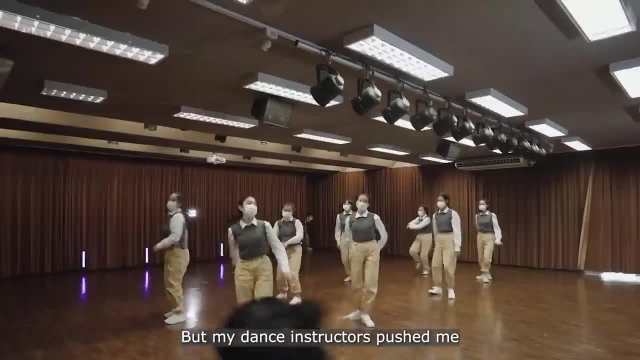 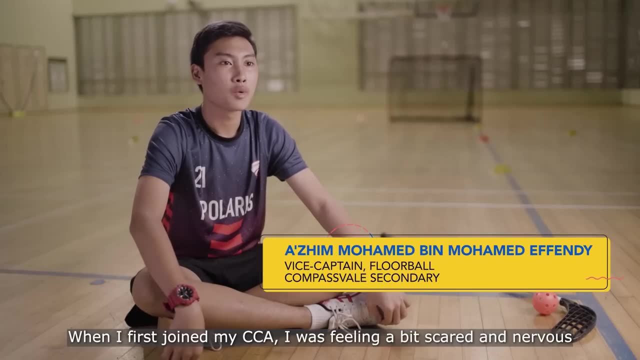 But since my teachers and my dance instructors, they pushed me and given me a chance to lead in this dance CCA. When I first joined my CCA I was feeling a bit scared and nervous because it's a new sport for me. Football has taught me to be more resilient and determined. 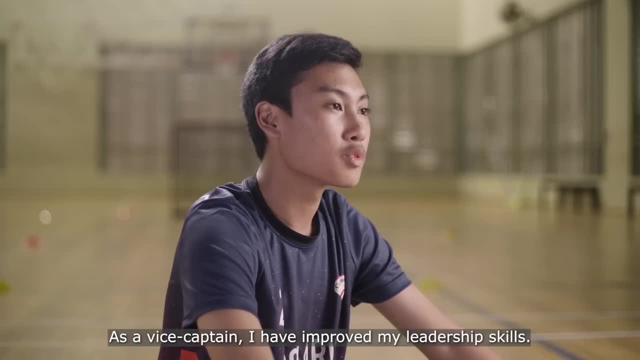 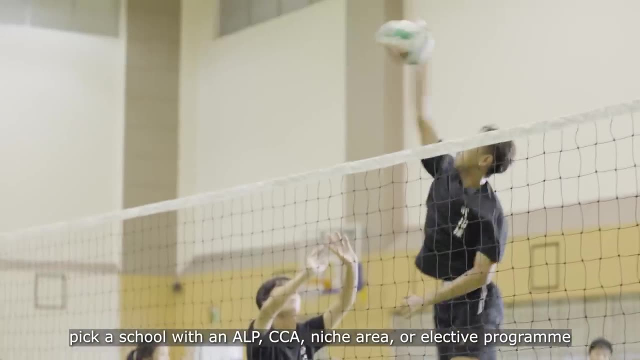 As a Vice-Captain, I have improved my leadership skills. If you are unsure of your strengths and interests, pick a school with an ALP, CCA, niche area or elective programme that you are keen on for you to explore further. 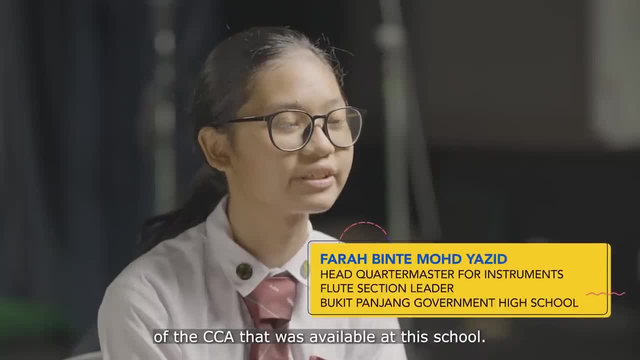 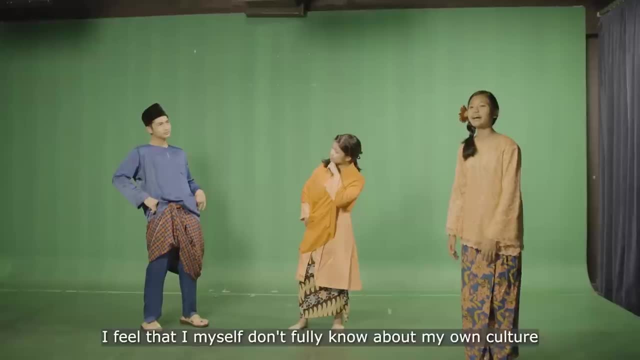 I chose to go to this school mainly because of the CCA that was available in this school. Another factor was because of the Malay Language Elective Programme that the school offered. I feel that I myself don't fully know about my own culture and wanted to fully immerse myself to understand it more. 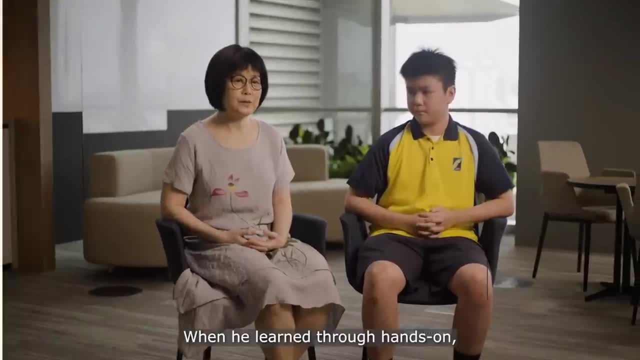 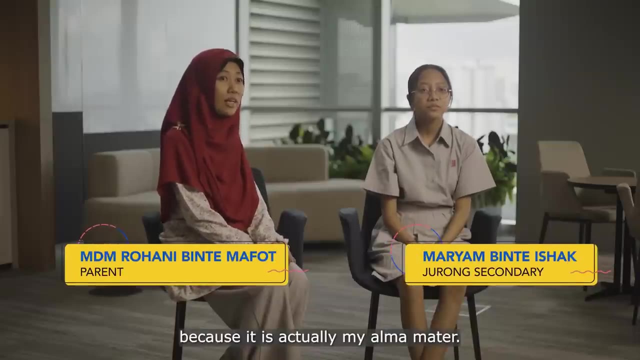 When he learnt through Hands-On he was able to understand the concepts better than through the traditional classroom learning. He became an independent learner. Mariam is in Jurong Secondary School because it is actually my alma mater. The teachers here are very caring and they have the students' interests at heart.